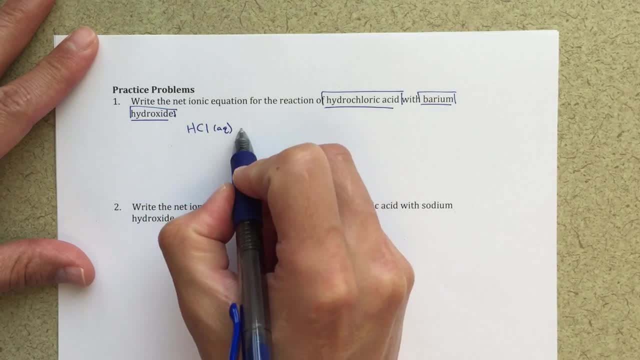 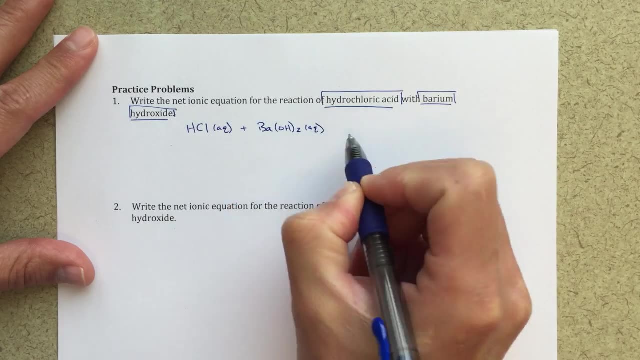 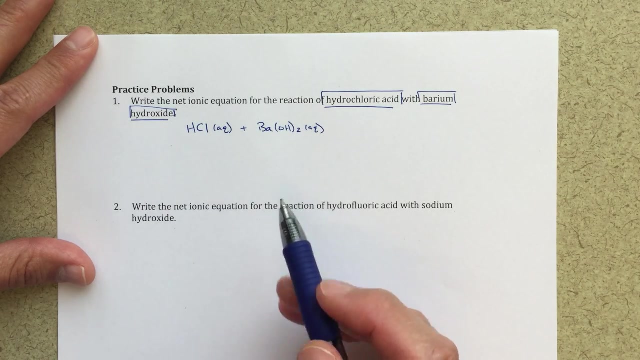 So I'm going to start by writing HCl aqueous, representing my hydrochloric acid, plus barium hydroxide aqueous- And again, I know both of those are aqueous simply because strong acid, strong base, My solubility rules tell me that barium hydroxide is going to dissolve completely. 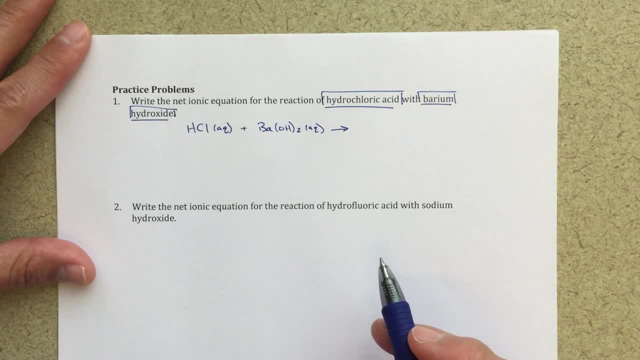 anyhow, Now for the products. this is going to be very simple. I'm going to write out a balanced molecular equation, So I'm going to start by writing HCl aqueous, representing my hydrochloric acid. this is a neutralization reaction. We need to start recognizing this is an acid. It helps that. 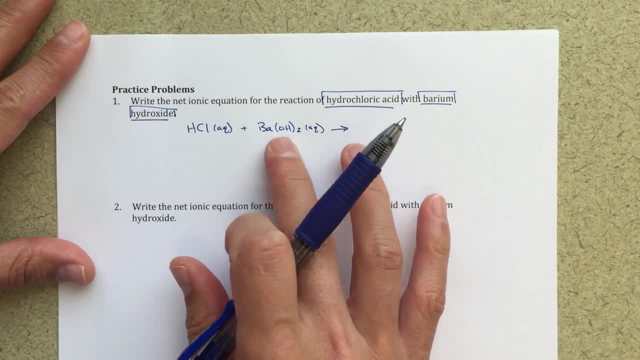 it says acid right there, right, But that barium hydroxide is a base. Anytime I see that hydroxide I want to be thinking base And I know that I'm going to form water as one of the products If 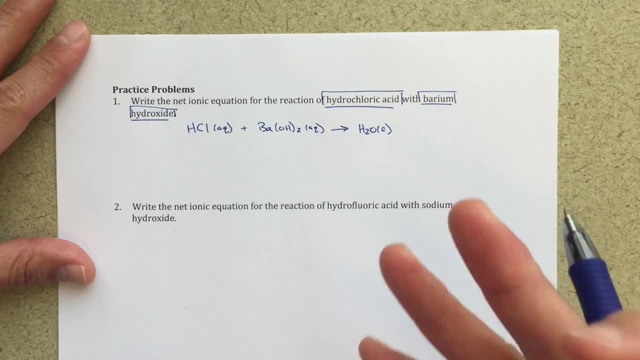 it's a neutralization reaction. if I react an acid and a base, we're going to form water. There's just no, you know no ifs, ands or buts about it. That's what's going to happen. And then, in terms, 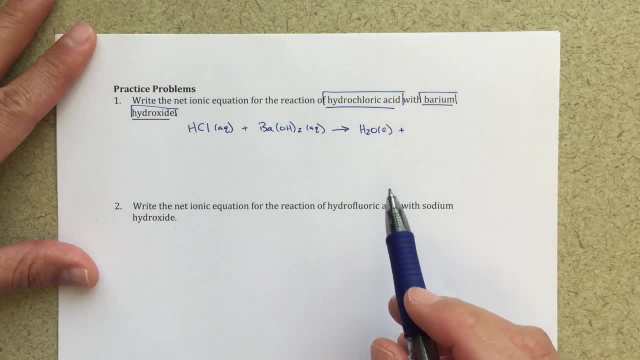 of figuring out what else is going to happen. I think there's a little confusion here and we're trying to sort of do too many things at once, So we're going to start by writing HCl aqueous, representing my hydrochloric acid. What we want to say is we want to say, well, what's left over? 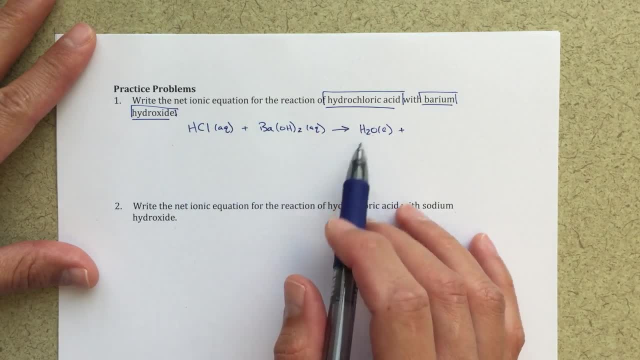 I've got a hydrogen here. I've got OH here. That's how I'm going to form the water. Then I've got barium and I've got chlorine and it's not balanced out yet. And that's okay, We're going to balance. 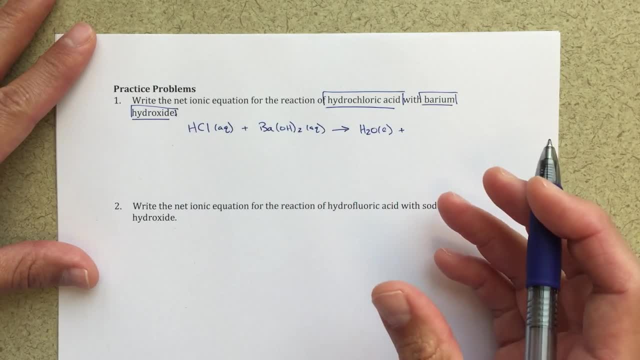 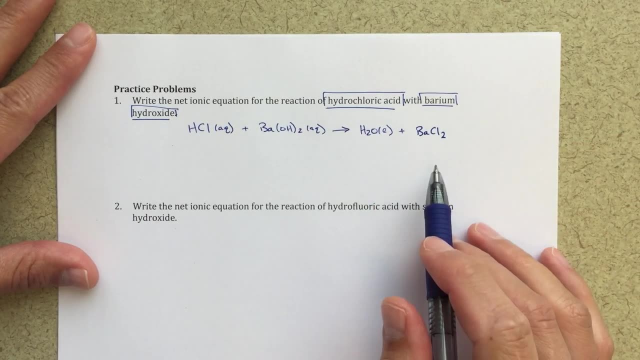 it next. But first I need to predict what the products are going to be and write those down. So I know it's going to be barium, Cl2.. So BaCl2, I've chosen Cl2 simply because chlorine is going to be the chloride ion minus one HCl. So I'm going to write that down And then I'm going to 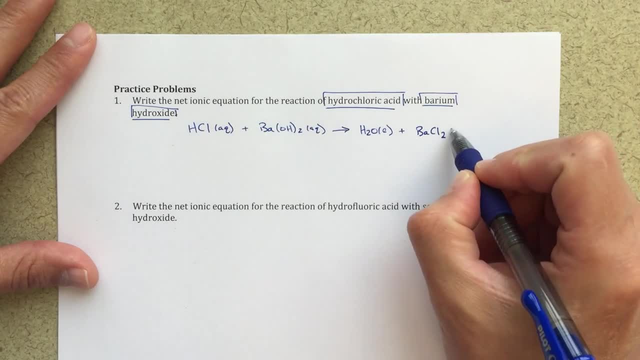 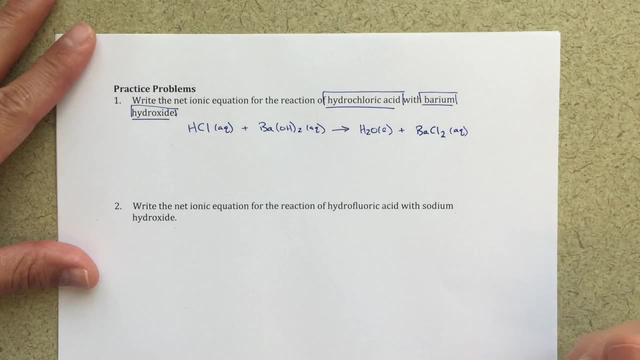 put a two plus charge. I need to balance it out. That's going to be a soluble compound. It'll be aqueous. You know, if I look at my list- chlorine halogens- those are going to be soluble. So this: 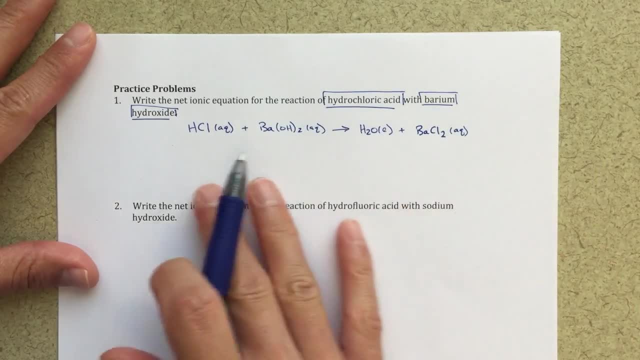 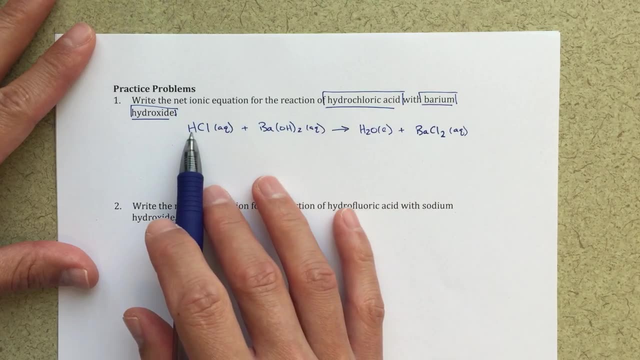 will be aqueous. Now step two: I'm going to balance this chemical equation. So when I balance the chemical equation, the way I would do this, I would look at the hydrogens first and say, well, I just have hydrogen here, I've got hydrogen here, I've got hydrogen here. It seems a little. 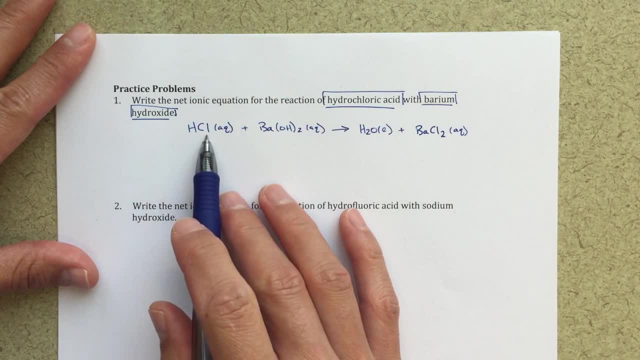 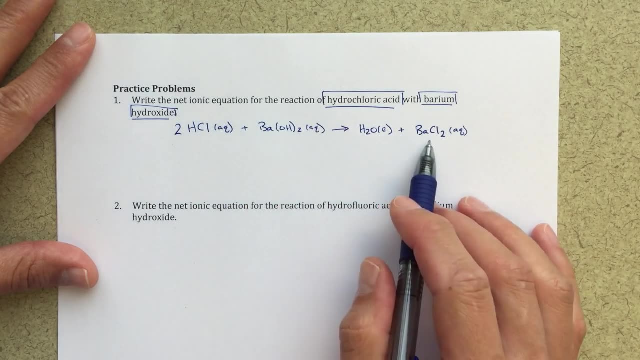 too complicated. I'm just going to skip hydrogen. first I'm going to go to chlorine. What I'm going to do is I'm going to put one chlorine here, two chlorines here. I'm going to need to put a two here. Now I'm going to go to barium. one barium here, one barium here. Let's do oxygen next. I've 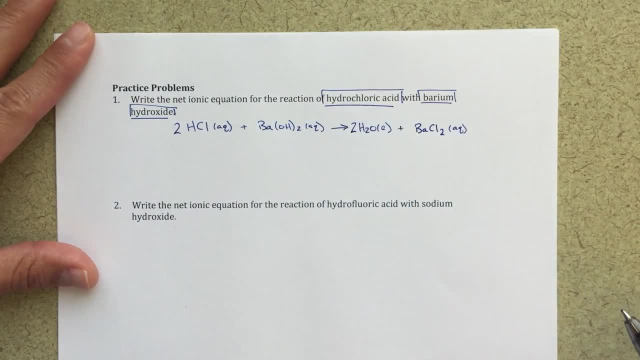 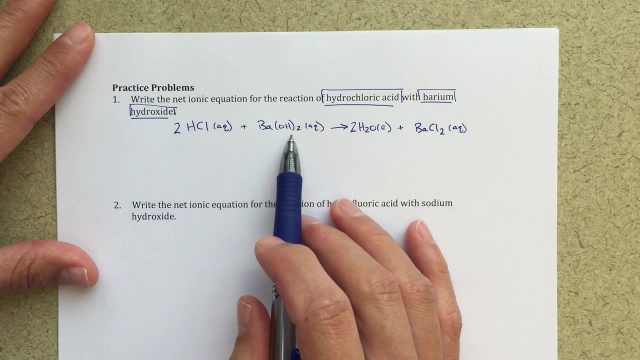 got two oxygens here, only one oxygen here, So we'll put a two in there Now, since everything else is balanced. now I'll look at my hydrogen and hopefully it'll already be balanced out. I've got two hydrogens plus two hydrogens is four, and I've got four hydrogens on this side. So this is. 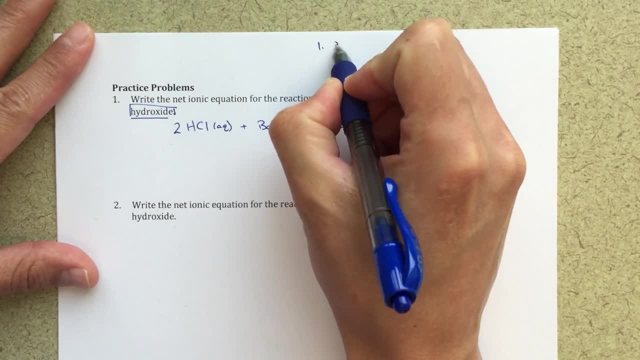 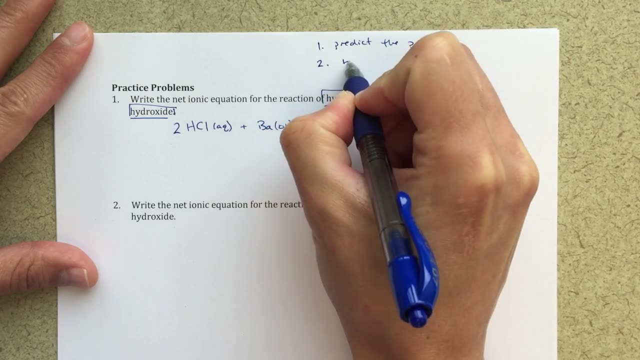 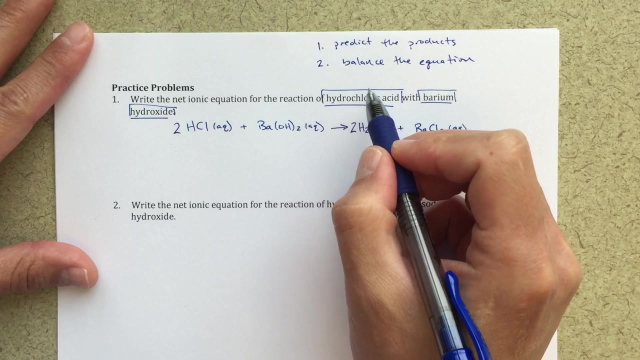 now a balanced chemical equation. So step one, predict the products And then step two, balance the equation. And I really want to stress this step two, worrying about balancing the equation, because I saw a lot of people today trying to do all of 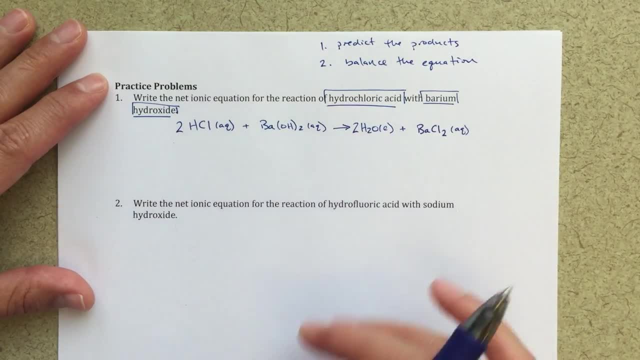 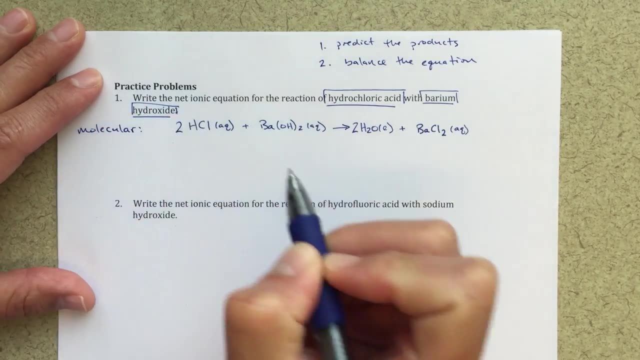 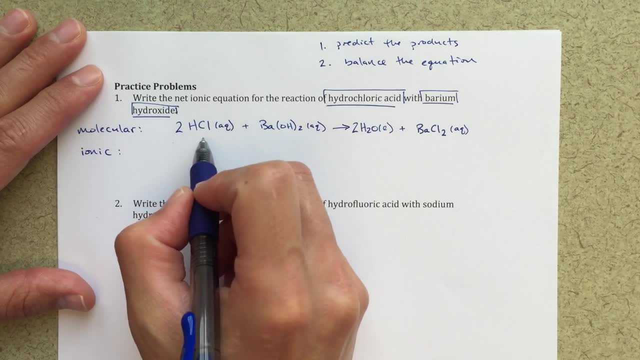 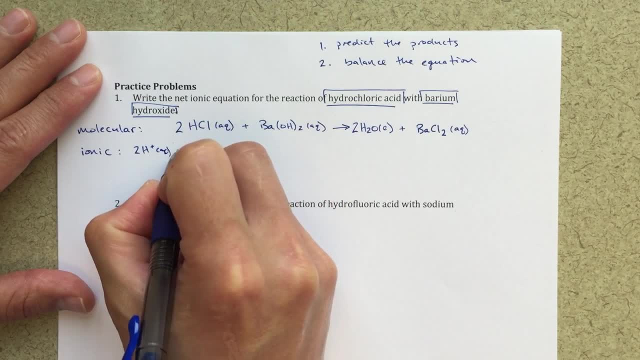 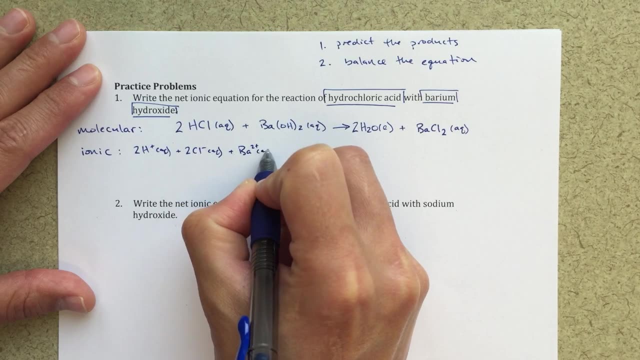 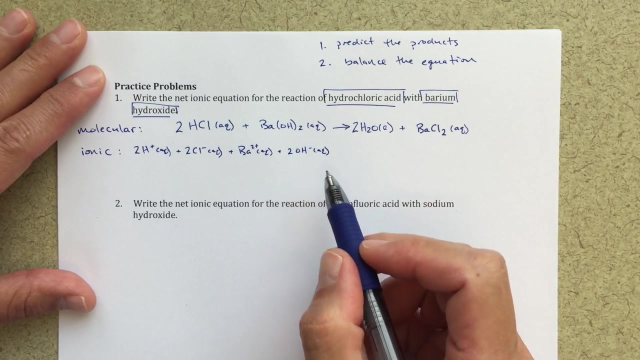 get two H pluses, since I've got two HCls plus two Cl minus plus barium, 2 plus plus two of these OH minuses, So it's OH2.. So two of those OH minuses That's all going to turn into 2H2O. 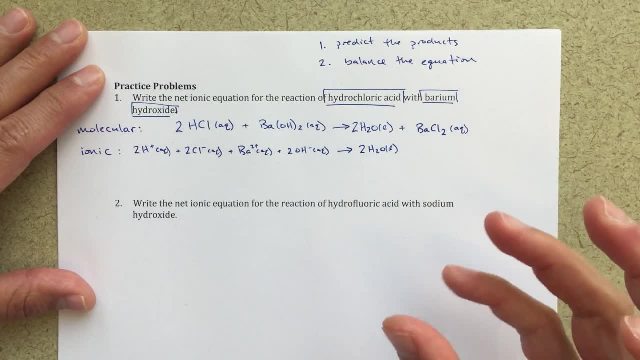 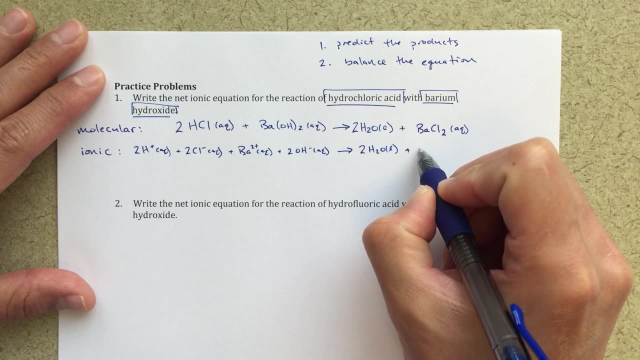 liquid. So H2O, it's a liquid. It's not going to ionize. So this will just sort of bring this down. We're not going to turn it into any ions Plus barium 2, plus aqueous, plus two Cl minus. 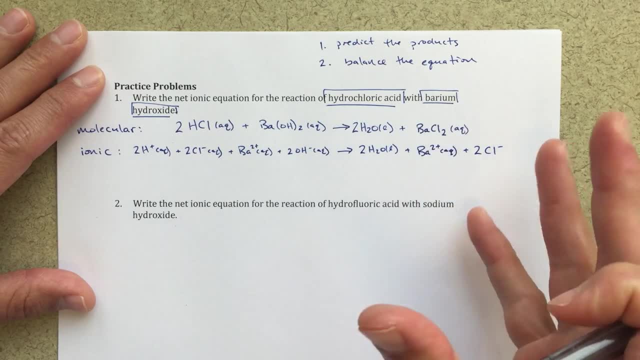 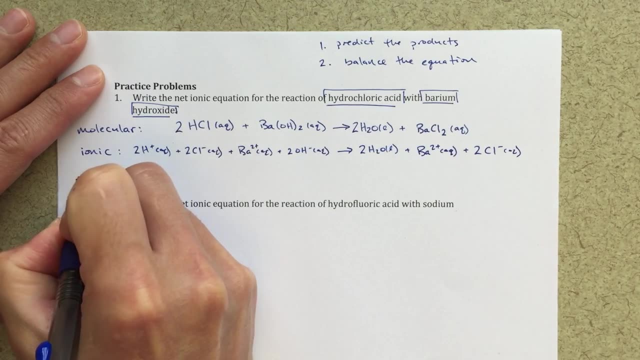 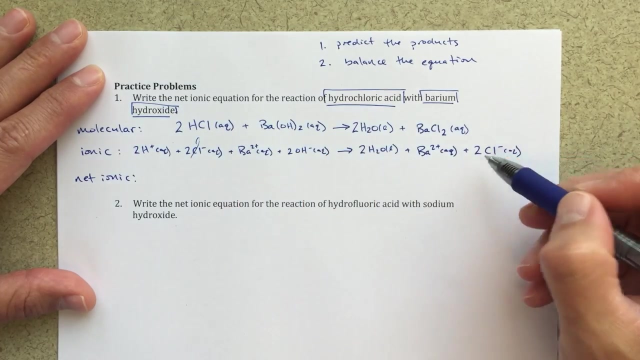 So again, even though it's Cl2 here that's going to dissociate into ions, I'm going to get two Cl minus ions, And that will also be aqueous. Now for my net ionic. that's going to be where I cancel out the spectator ions. So I see chlorines on both sides. 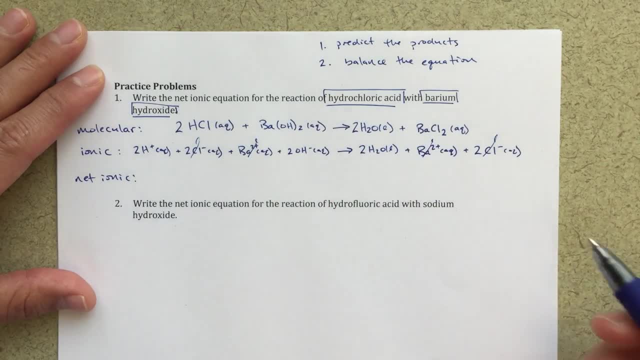 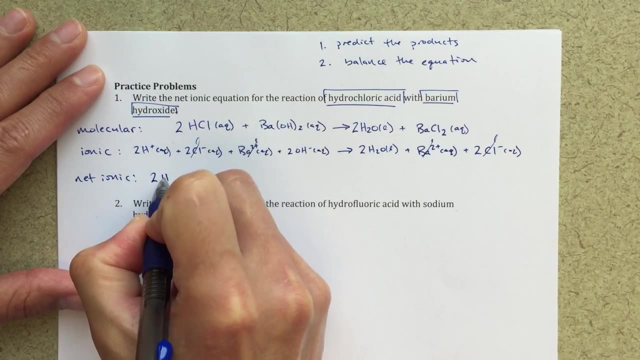 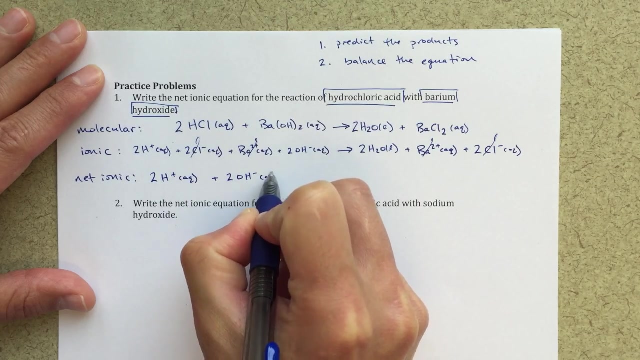 I see barium on both sides, And that's all my spectator ions. These are spectator ions. They're just watching the reaction occur. So for my net ionic equation, we're going to end up with two H plus plus two OH. minus reacts to form two H2O liquid. Now a lot of times what we're going. 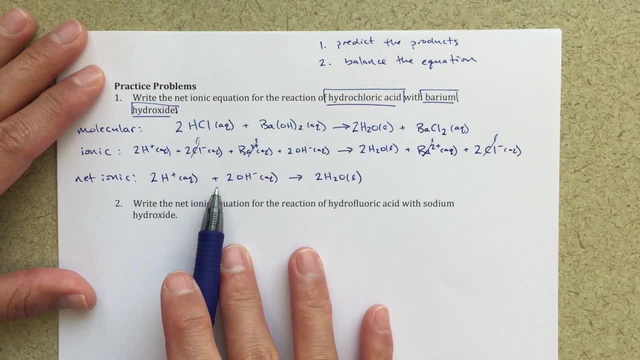 to see is that we're going to get two H plus plus two OH minuses, So we're going to get two H2O liquid, And what we're going to see is people simplify this even further. So since we've got two, two, two as our coefficients, we can really rewrite this as one one one. I'm okay with us. 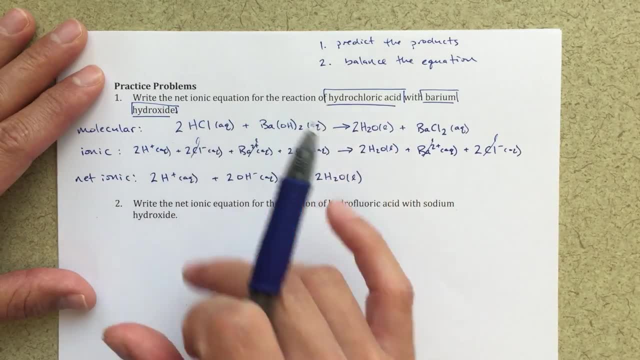 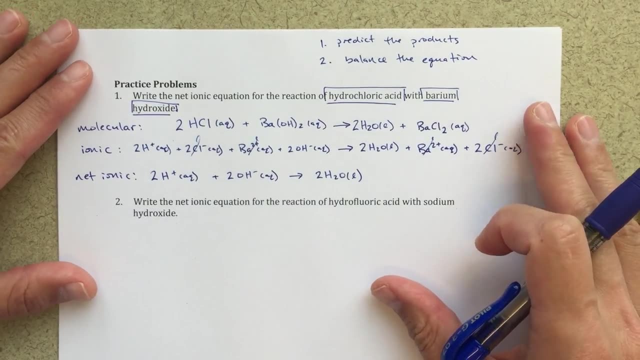 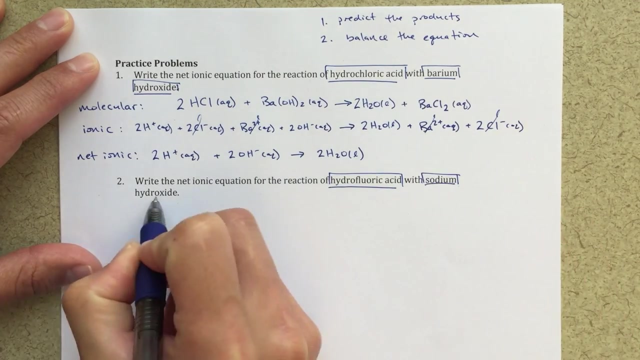 leaving it this way. I think it makes a lot of sense. It comes straight from our molecular equation. So if you left it like this, I think that's a-okay. I'm okay with that. All right, let's do the next one And the next one. I'm using hydrofluoric acid with sodium hydroxide. 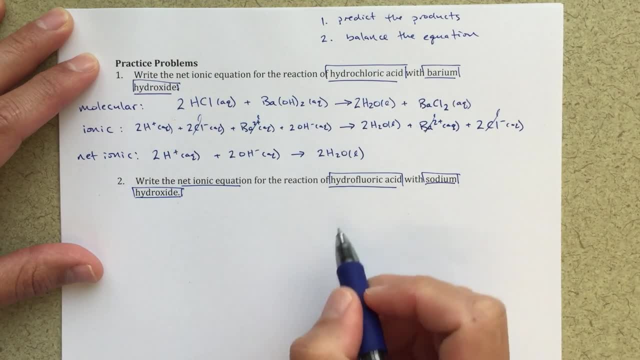 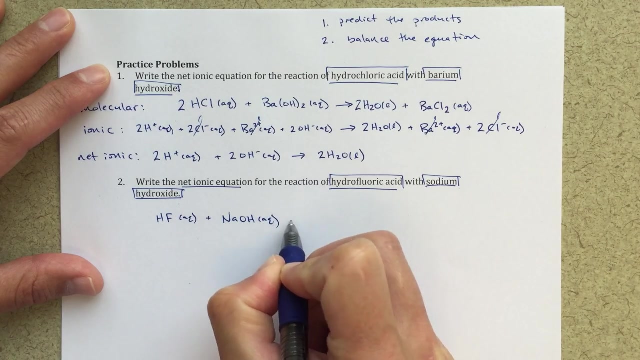 And again I'm looking for that net ionic equation. So I know hydrofluoric acid is HF. I'm going to write aqueous because we're going to be, you know, doing this in in water solution: chemistry plus NaOH, aqueous. Right away I've got an acid, I've got a strong. 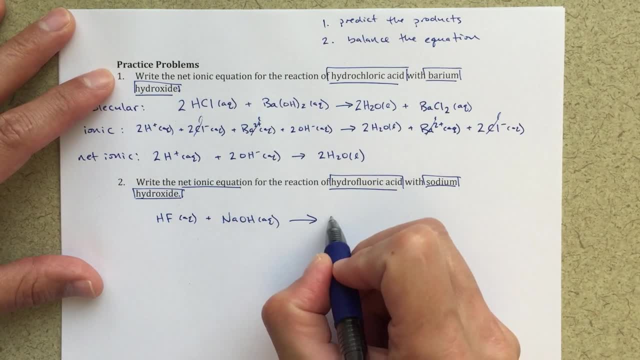 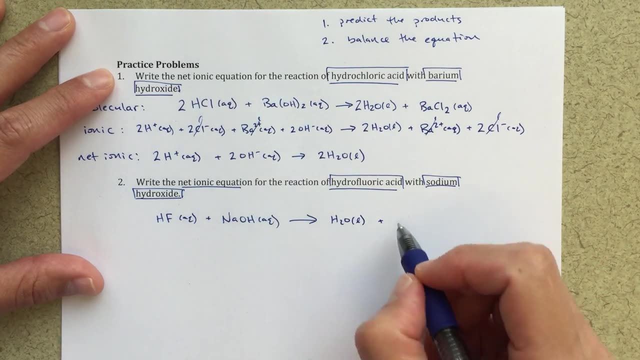 base. I recognize sodium hydroxide as a strong base, So I know I'm going to form water. right, I'm going to form water right away, It's my neutralization product- And then I'm going to form sodium fluoride. So I'm sort of just taking what's left over and 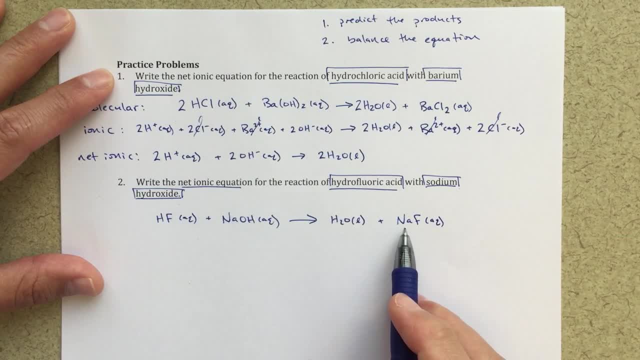 saying: well, I'm going to form sodium fluoride. That will be aqueous. Anything that is dissolved and has sodium in it will. anything that has sodium in it will dissolve. right, It's our first solubility rule And this is my molecular equation. If I want to write my ionic equation. 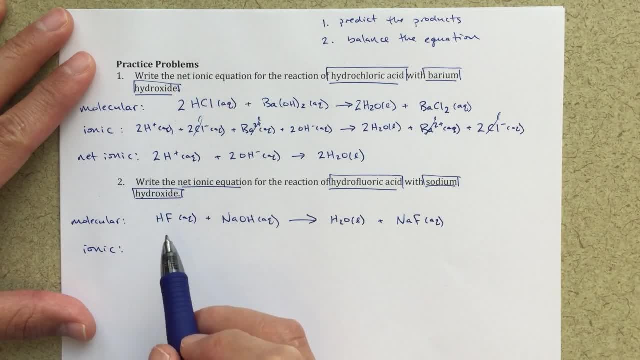 now here's where it gets a little confusing with HF. HF is a weak acid. Since HF is a weak acid, it will not ionize. It will not break into H plus and F minus, really that much, So it will a tiny.